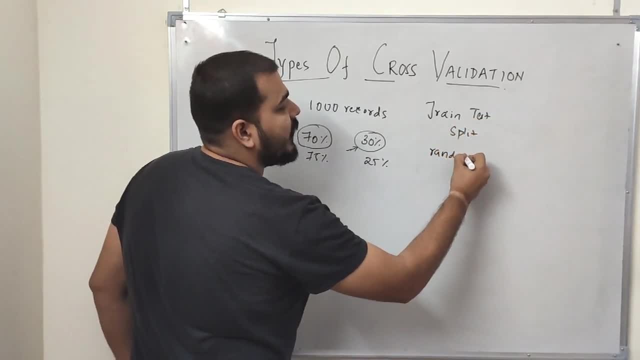 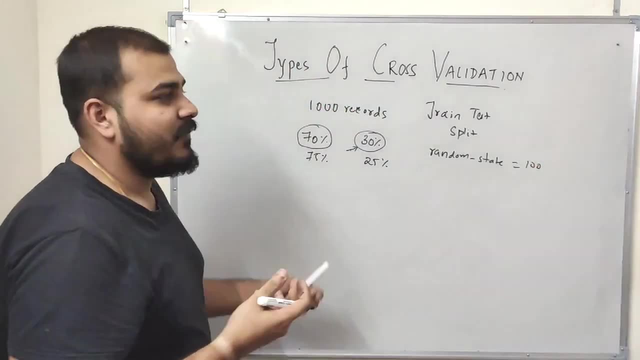 We usually use a random state random state variable. It will be like this only in random state variable, and we define this random state, anything you can define: 100,, 200,, 5,, 10,. Now, based on this random state, what it does is that it randomly selects the data point. 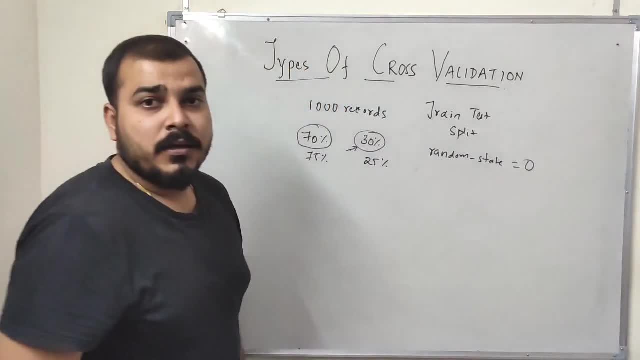 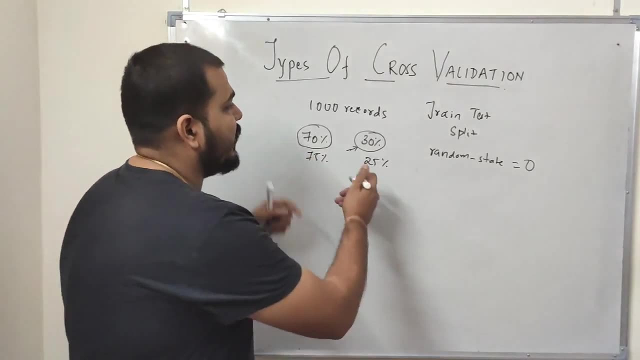 Now suppose I have selected random state as 0. Okay, Now when I select the random state as 0 and I say that: okay, do that 70% and 30% split Right. And when we take it and suppose the accuracy is somewhere around 85%. 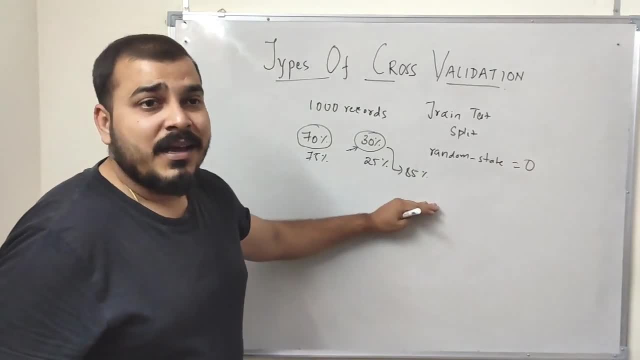 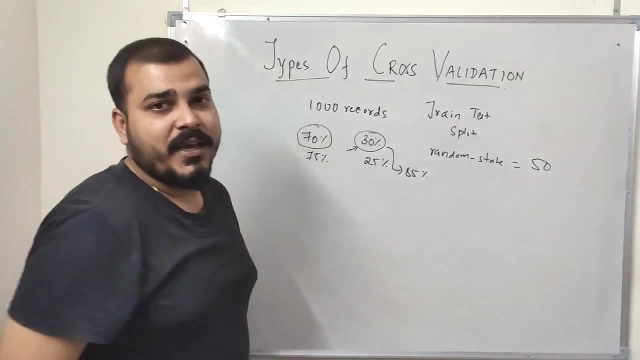 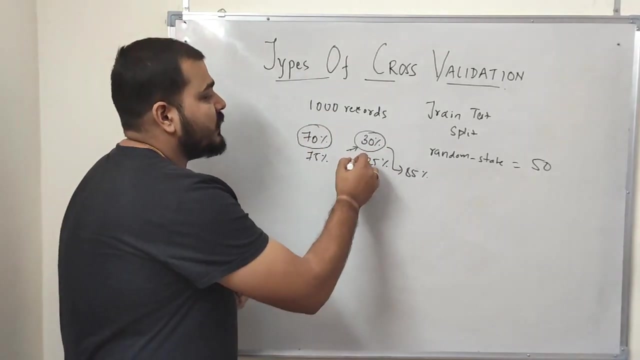 Okay, Now, when this accuracy comes to us as 85%, Now what I will do is that again, I will try to perform this random train test split with different random states. Suppose I select 50 now. Now, when I do this again, this will get shuffled, This will completely get shuffled, And then you will be seeing that suppose, in the next experiment, when I selected, the random state is equal to 50. I got an accuracy of 87%. 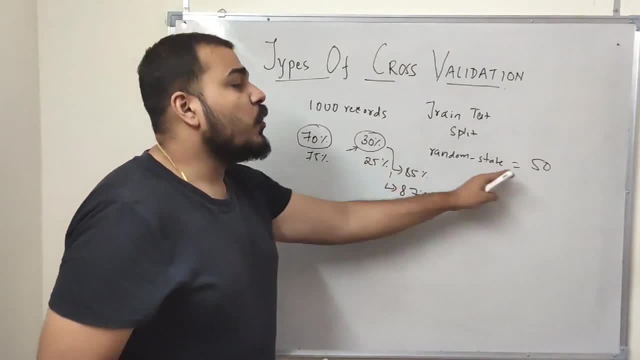 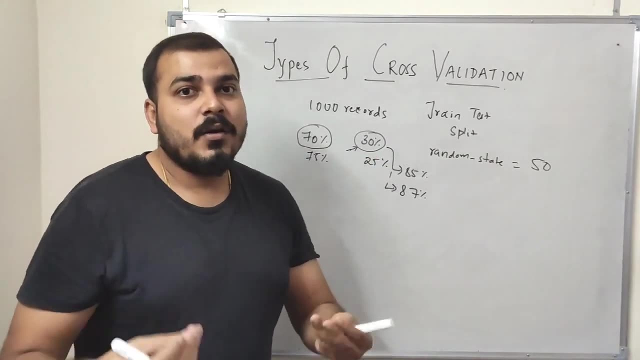 So the main point: you need to understand that if I go on selecting different, different random state, your accuracy fluctuate, Right, So you won't be able to tell your stakeholders what accuracy your model is exact, Right, What exact accuracy it is basically given. 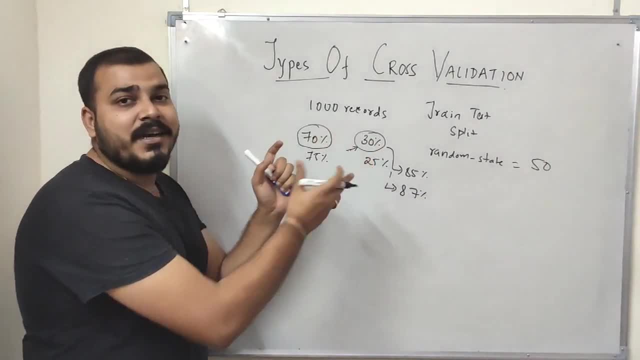 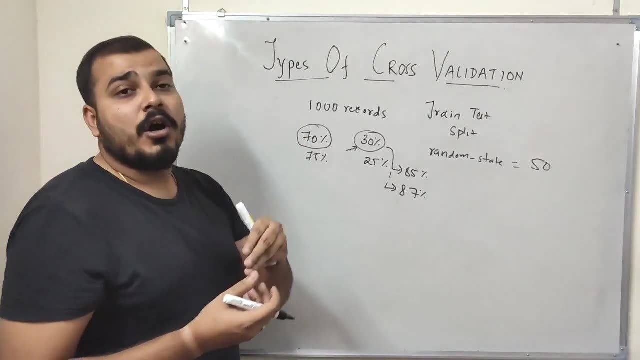 Because as the random state changes, Your training and test data is basically changing. And when that particular training and test data basically changes, at that time when you train your model, What will happen? Your model will actually be fluctuating, your output Right And so your accuracy changes. 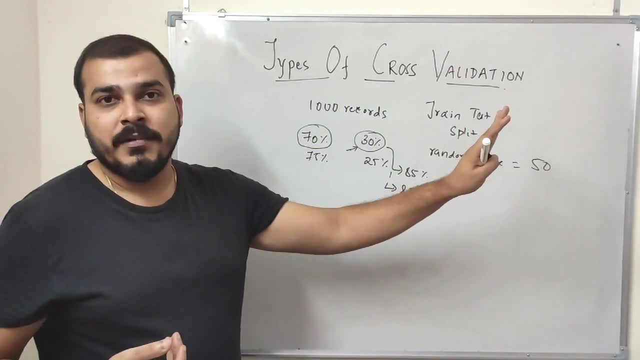 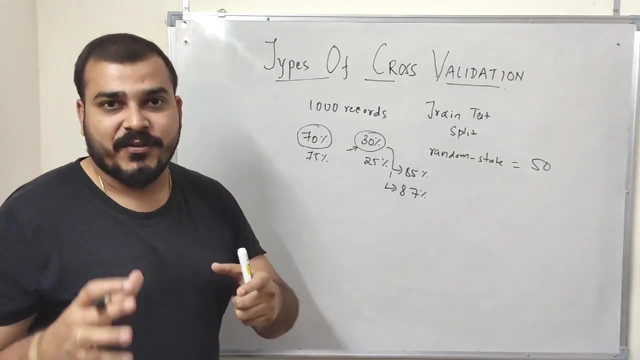 So, in order to prevent this, we have a concept called as cross validation. Now, in cross validation, what is the simplest rule in that I will just discuss by discussing the various types first. So let me rub this and let me just tell you what are the data types. 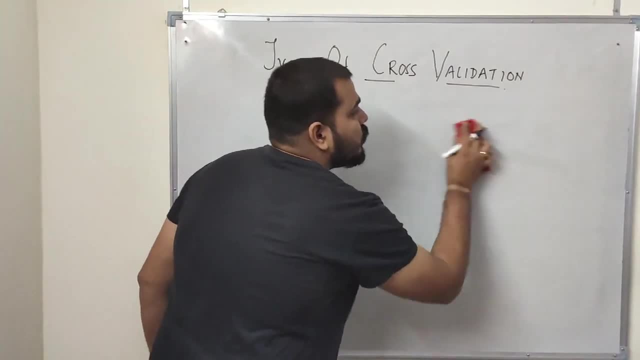 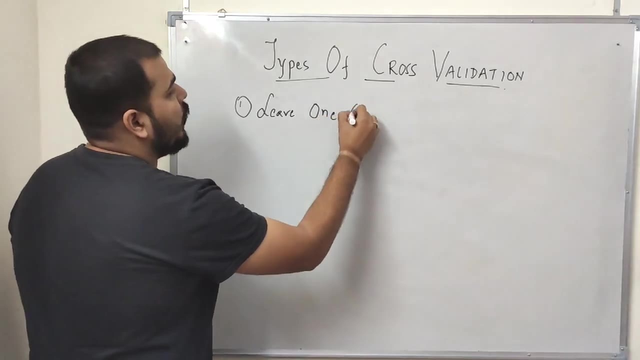 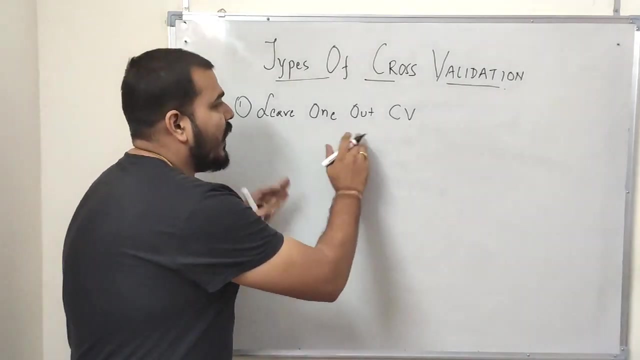 So let me just tell you what are the different types of cross validation. So the first time Is something called as leave one out cross validation. Now you may be thinking, OK, This is just like leave one out. We also say it as L O O C, V. 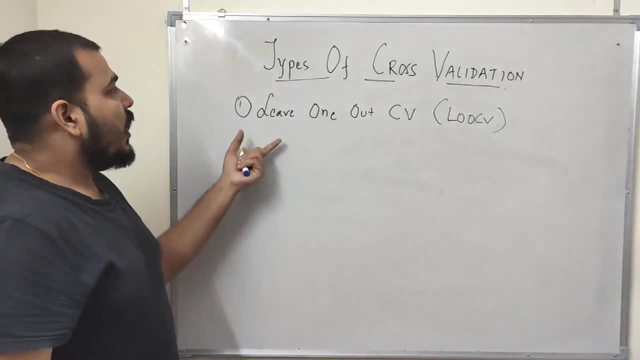 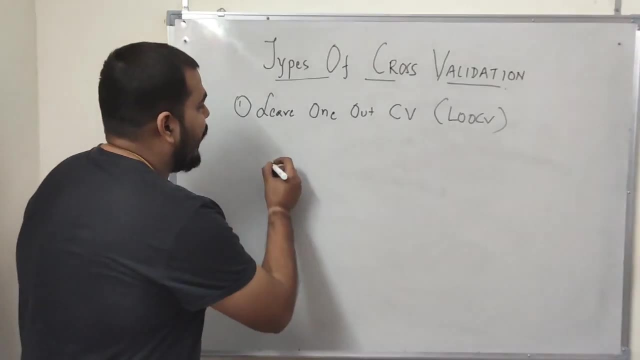 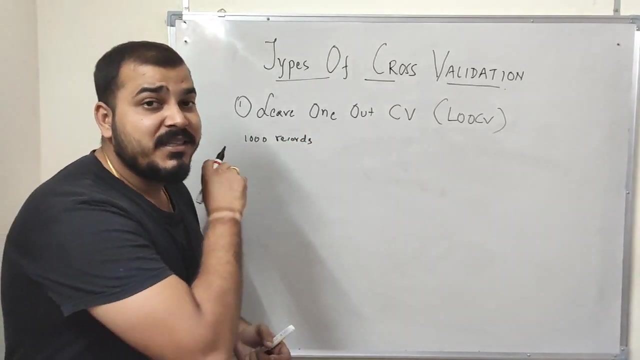 OK, So this is the short form, But in short it is basically called as leave one out cross validation, So how this particular cross-validation works. So first, what will happen is that suppose I have 1000 records. Now, when I say 1000 records, that basically means data points. 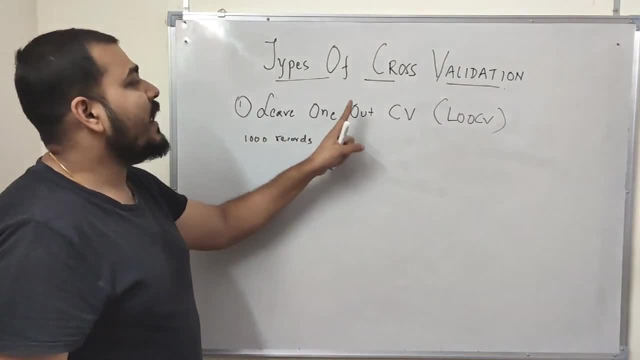 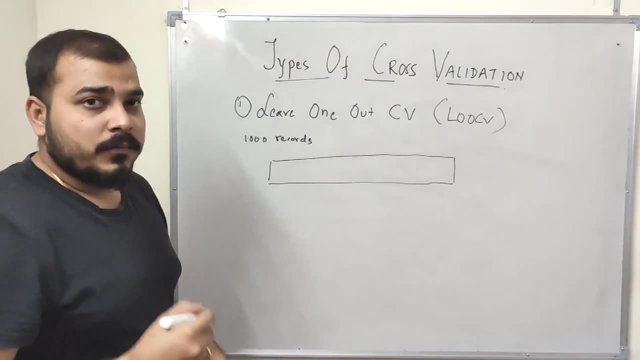 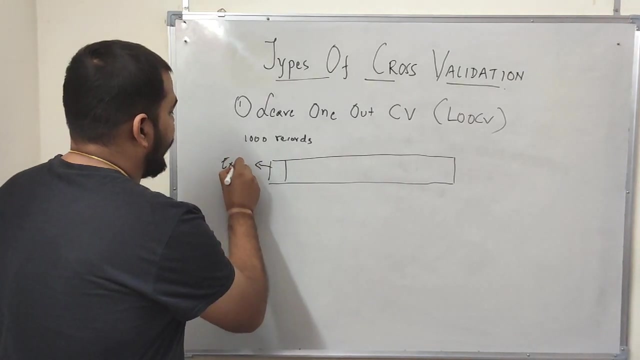 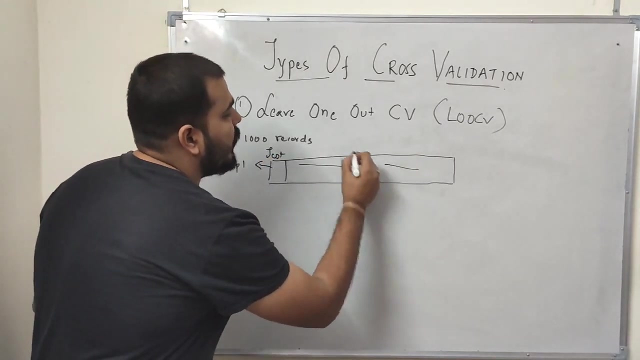 Now, in this 1000 records, the leave-one-out cross-validation basically says that the rule is like: from all these 1000 records I will take one data set at a time. Suppose this is my experiment 1.. So I will take this one data set as my test and remaining all will be my train. 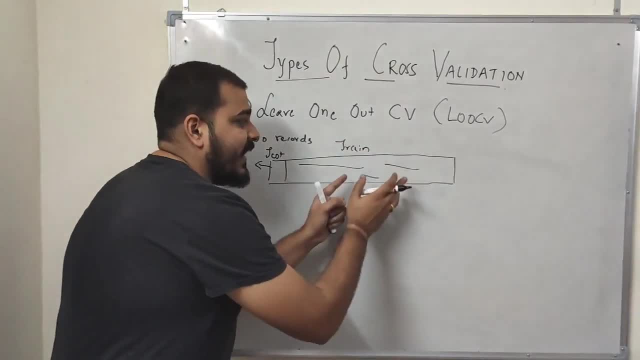 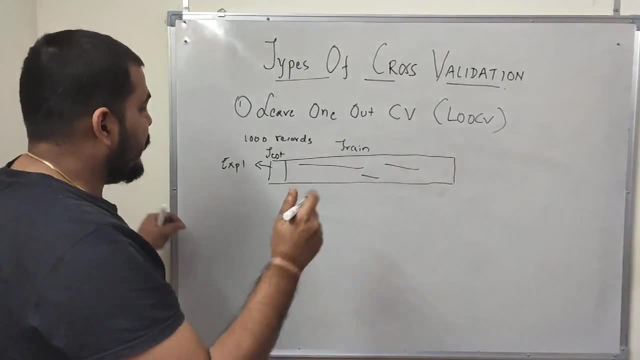 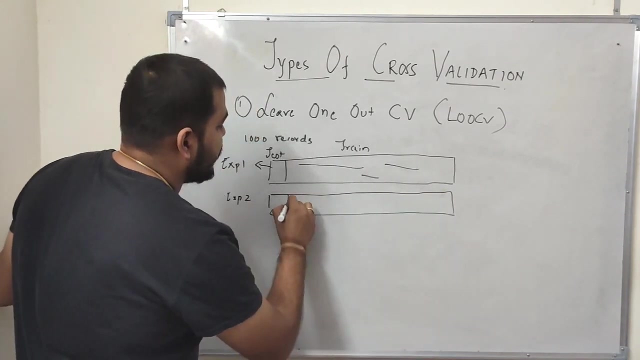 Now, based on this, the model will get trained onto this particular data and it will be tested on this one single data. Now, similarly, in the experiment 2, what will happen? The next data will be your test, And this is simple. This is just one, guys. 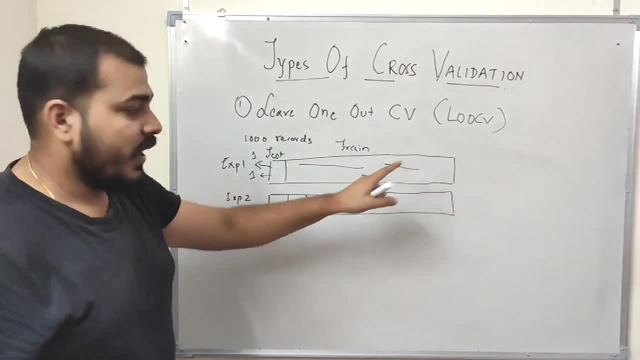 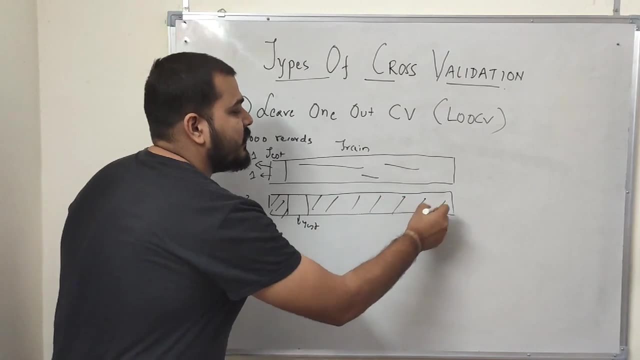 This count is only one because leave one out. So next, second one data will be your test and remaining all will be your train. That basically means this will be one and remaining all- 999- will be your test data. And again the same process is continued. 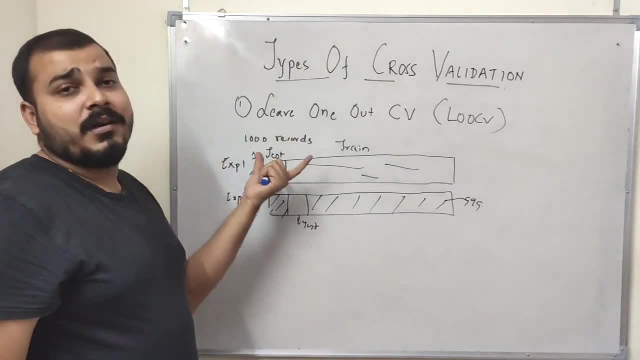 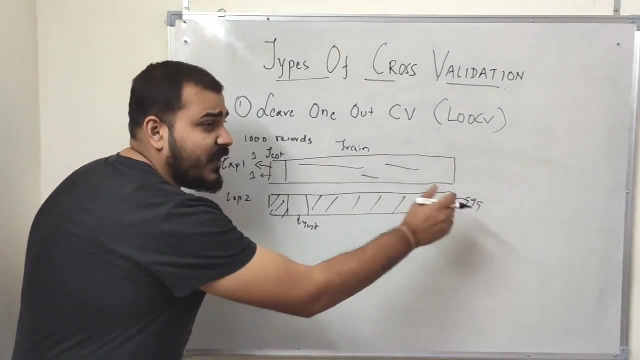 Now just understand, guys: if you are just taking one record for 1000 records, what will happen is that I have to perform many iterations. That basically means that if I want to cover each and every data set, I have to run 1000 iterations. 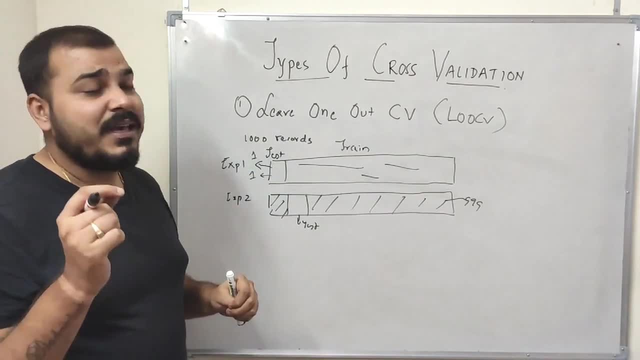 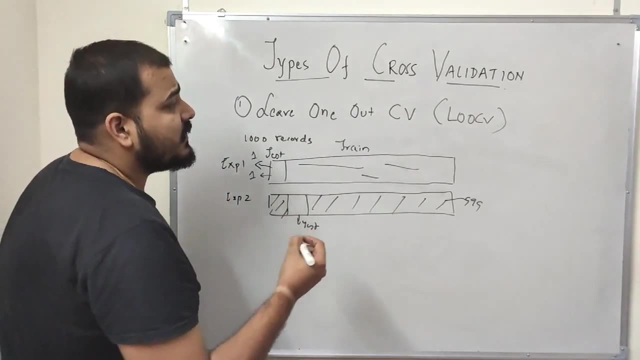 Now just understand how much computation power is there. That is one disadvantage of leave one out: cross validation. Let us discuss more disadvantages. First of all, you have to run many iterations and this will lead to low bias. The second disadvantage is that it will lead to low bias. 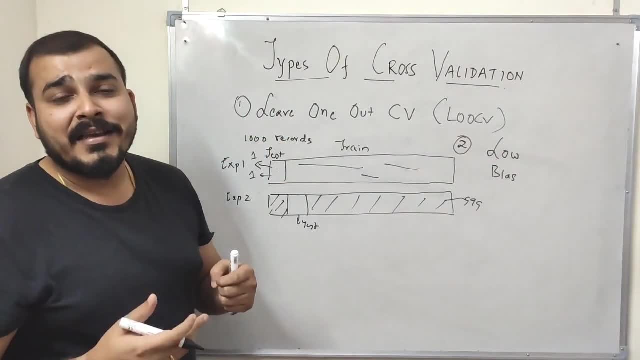 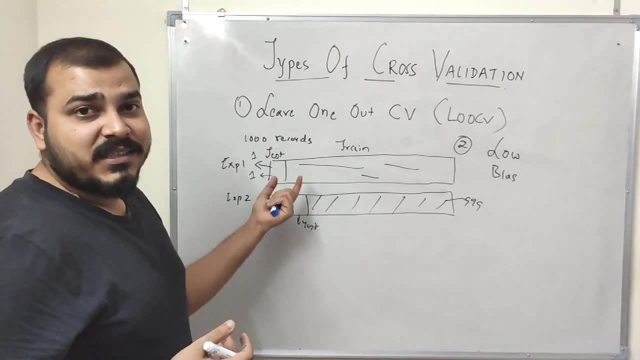 Now, what is low bias? I hope I have discussed already what is a high variance, high bias, low bias. Low bias basically means that for the training data set and this test data set, you are getting better result. So over here you can see that for the training data set. 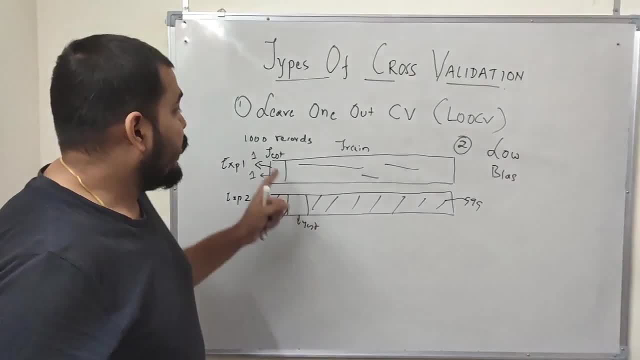 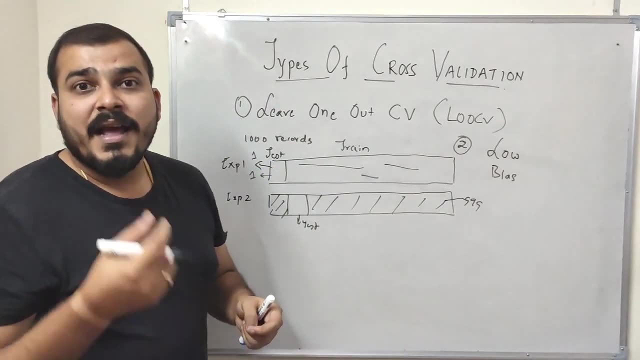 it will be like basically like a high variance kind of stuff. But whenever a new test data come, whenever the new test data come, when we try to deploy this model into the production, at that time the accuracy will go down, The error rate will become high. 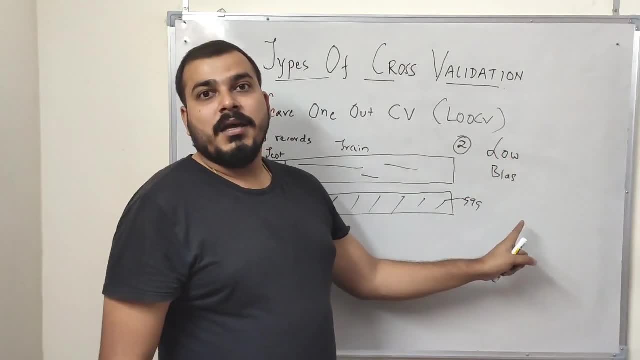 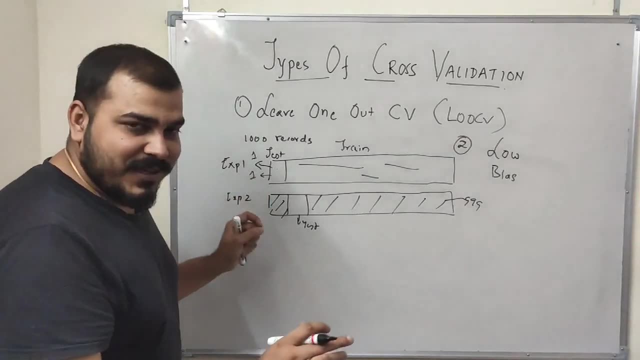 That is what this low bias condition says. So two problems with leave one out cross validation. This was used long back. Nowadays nobody is using this, So I needed to tell you what are different types of cross validation, so I am mentioning this. 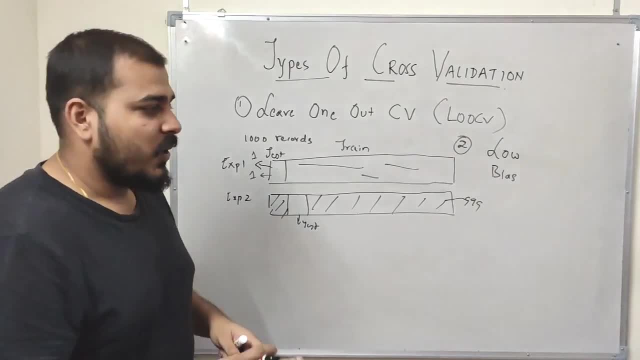 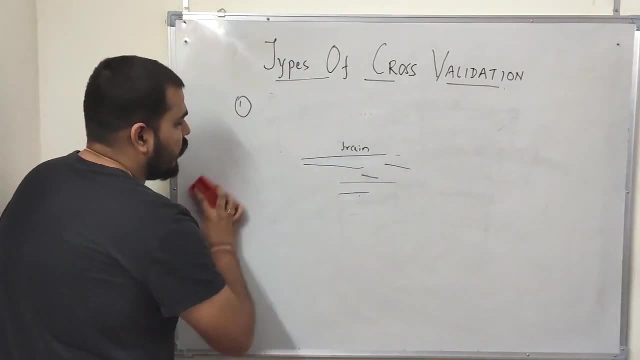 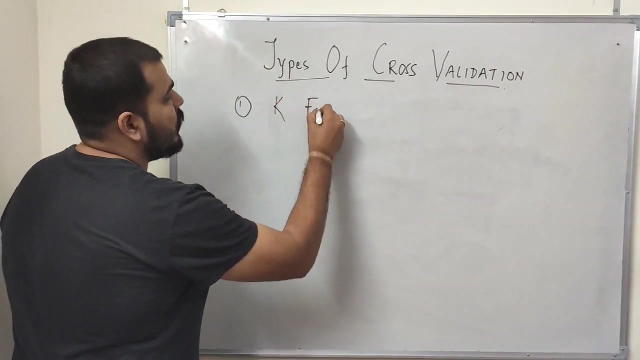 Not so important and nowadays nobody is basically using it. Now the second type, which is the most common and many of them are using, is called as K-fold cross validation, So I will just write it down. So this is my K-fold cross validation. 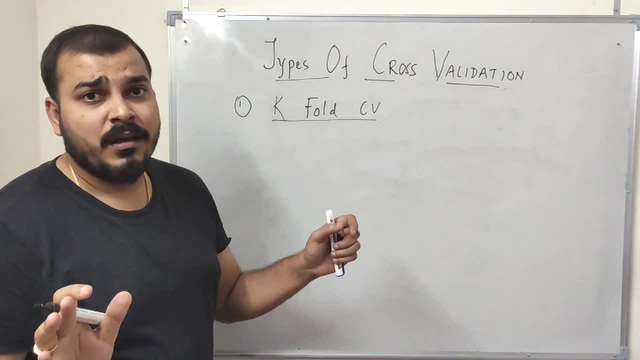 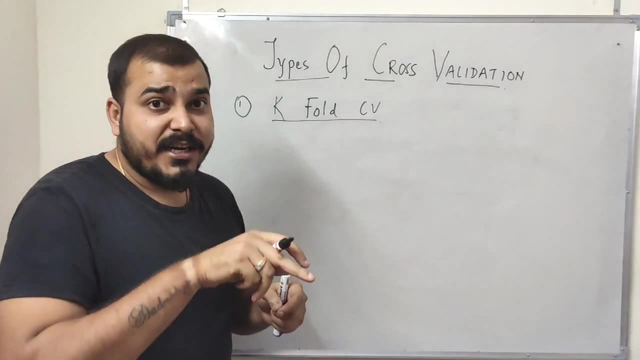 Now in K-fold cross validation. it is pretty much simple, very easy, just to understand. Now see, try to understand- the disadvantage of random state, Sorry, disadvantage of train test split Over there. whenever you change the random state, your training and test data changes right. 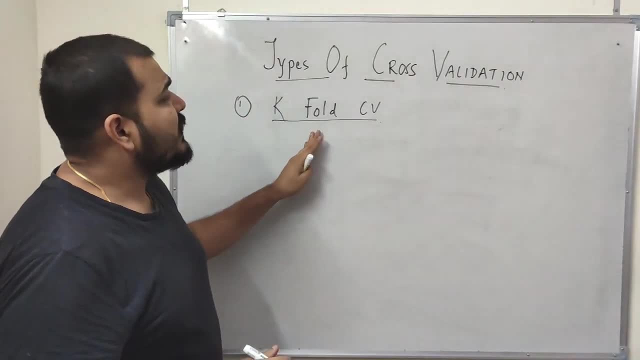 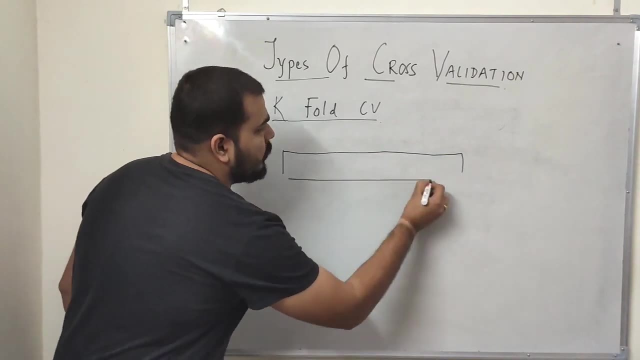 Because they are randomly selected. So, in order to do that, what we do is that we use K-fold cross validation. Now, in K-fold cross validation, suppose your data set is 1000 records. Suppose this is your 1000 record. okay. 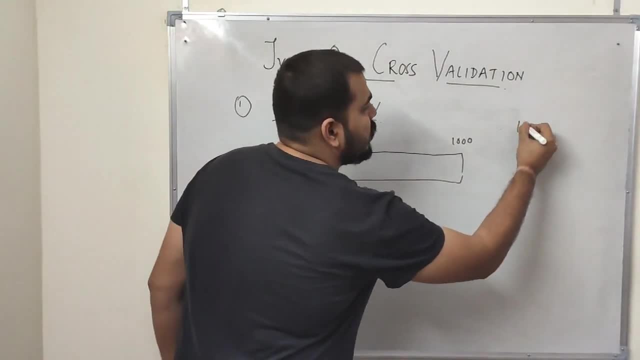 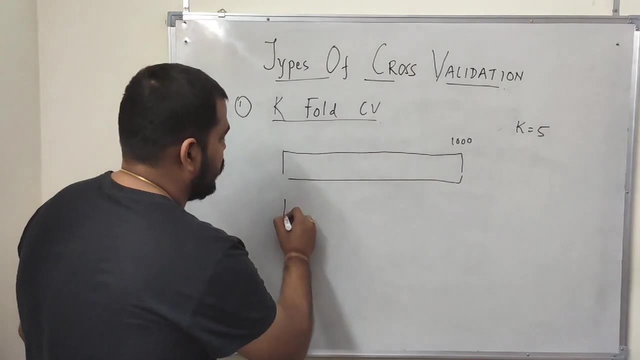 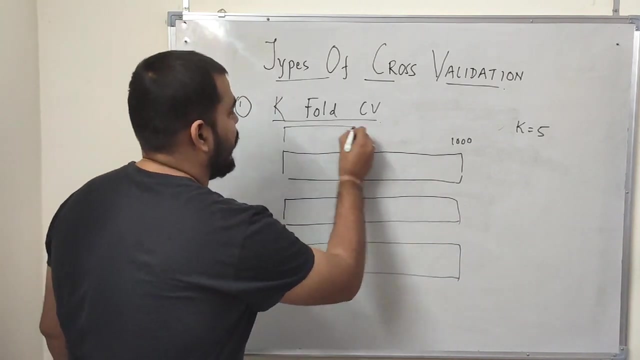 Now we select a K value, Suppose I say K is equal to 5.. Now this K basically means 5 experiments: 1,, 2,, 3, suppose over here 4, and this is my 5th. So this 5 experiments, it will say: 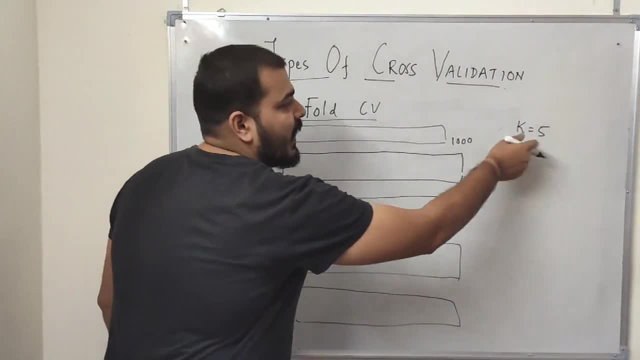 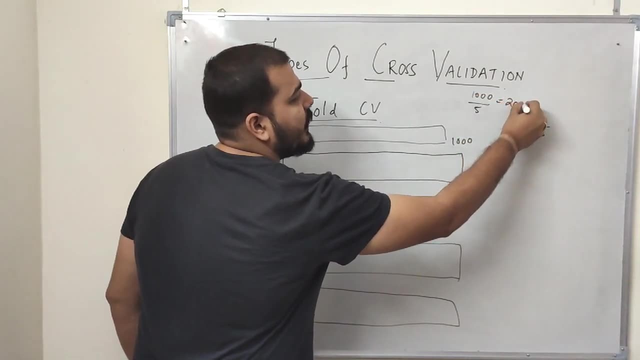 For each experiment, it will decide, based on this K value, what should be the test data. Now, when I divide this- 1000 divided by 5,, that basically means how many data will be there- 200 will be your test data, So the first 200 will be your test data. 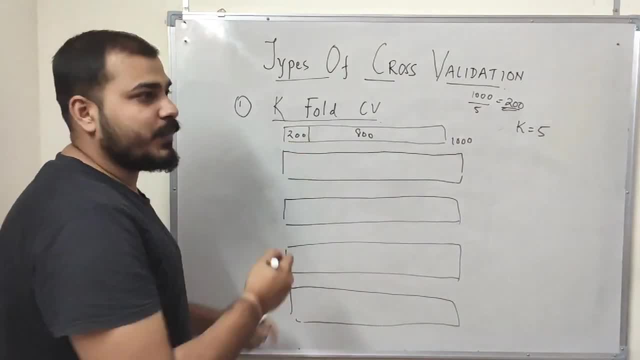 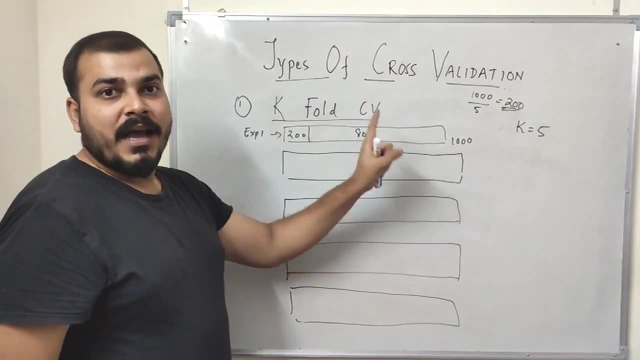 The remaining 800 will be your training data In the first experiment. this is my experiment 1.. So this model will get trained on this 800 data set And then it will be tested on 200 data set And we will be getting our accuracy 1.. 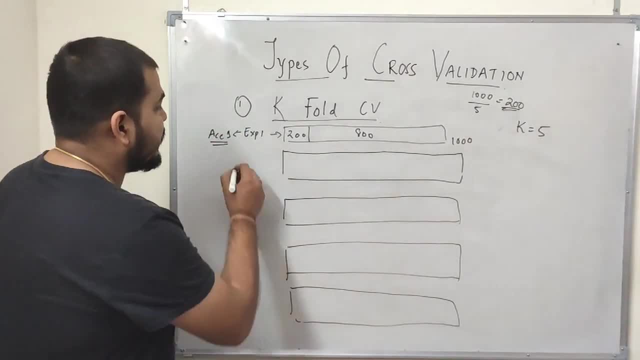 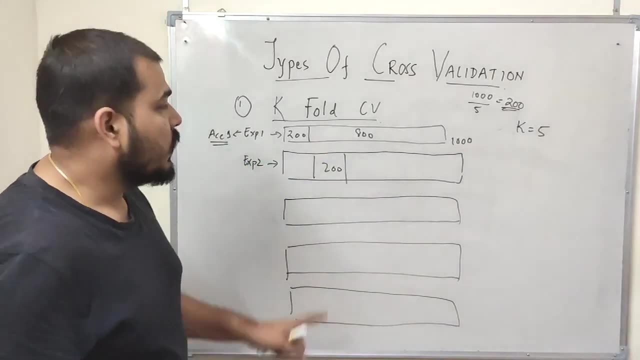 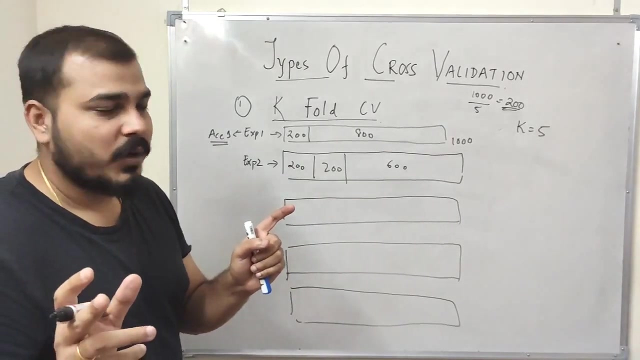 Suppose this is my accuracy 1,. okay, In the second experiment, what will happen? The next 200 records will be your test data And then this 600 plus this 200 will be your test data. okay, Sorry, this will be your test data. 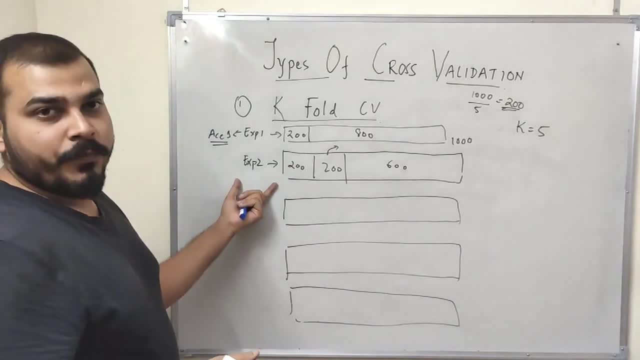 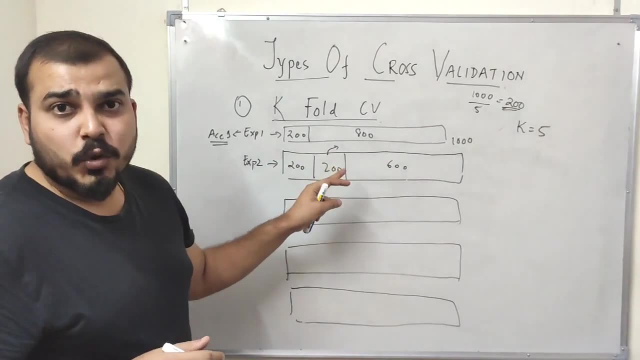 And this 600 plus 200 will be your training data in the experiment 2.. So the model will get trained on this 600 plus 200 training data set And then it will be tested on this 200 data set, which is your test data set. 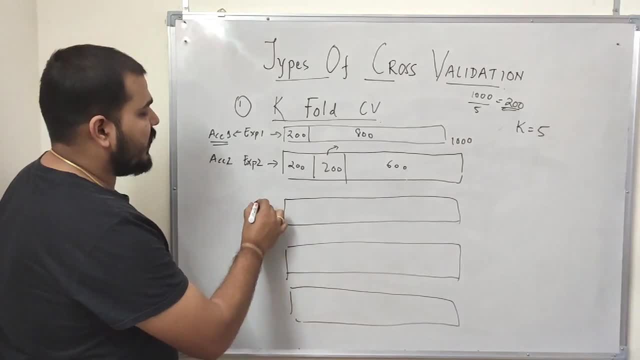 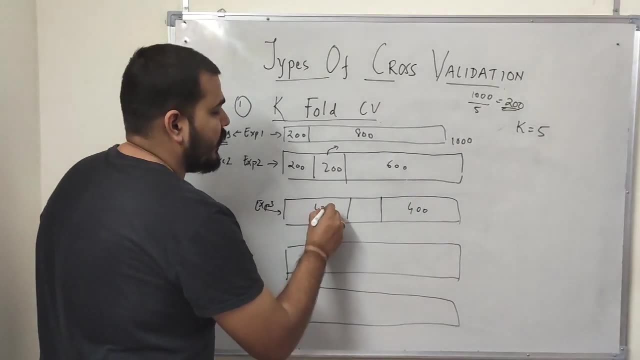 And again it will give you an accuracy: 2. Now, similarly, in the experiment 3, what will happen? The next 200 data set will get selected And again, here you will have 400.. Here you will have 400.. And this will be your test data set. 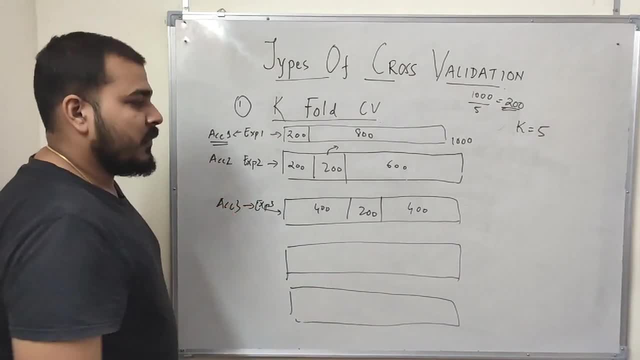 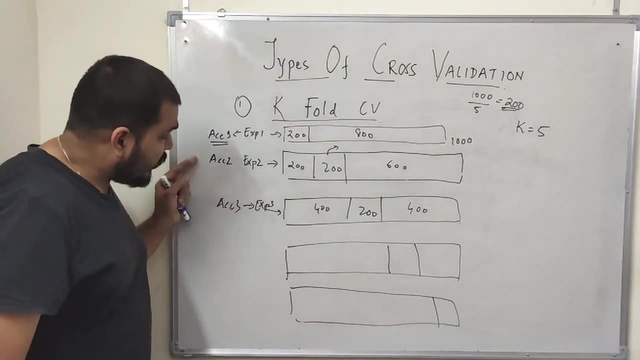 Again, the model will get trained and you will get an accuracy 3.. And this will continue unless and until the whole iteration is completed. Now, finally, you have accuracy 1,, accuracy 2, accuracy 3, accuracy 4, accuracy 5.. 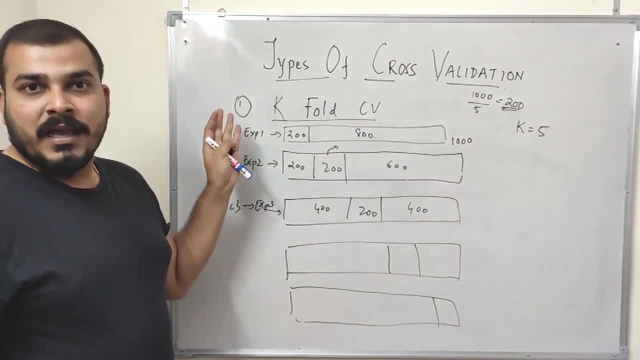 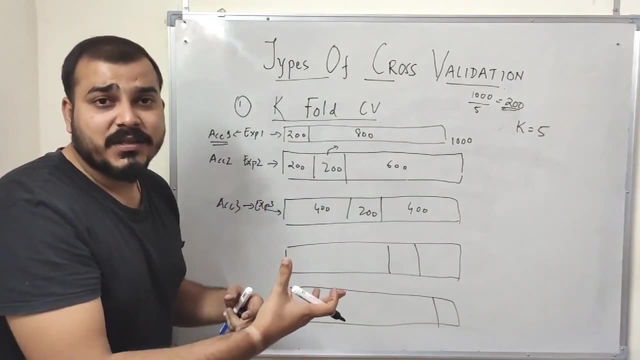 What you can do is that you can find out the mean of this accuracy And then you can take your tell your stock Stakeholders basically, that this particular data science project or machine learning use case is basically giving you an average of this accuracy after applying k-fold cross validation. 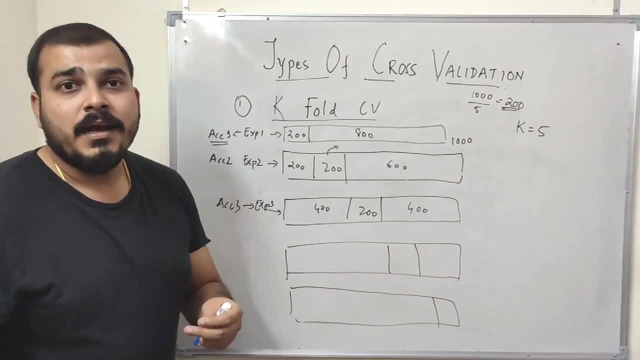 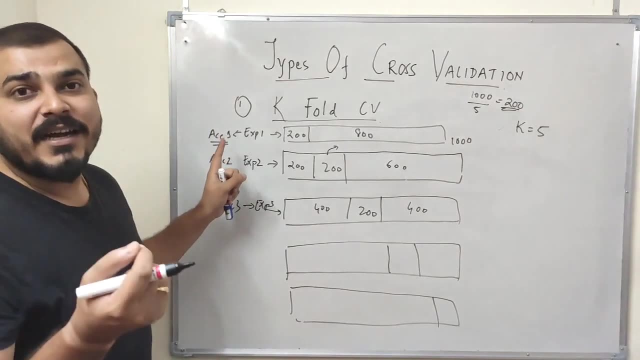 Sometimes you can also say your stakeholders right That the minimum accuracy that you can get with respect to this model will be the minimum of this particular all the accuracies, And the maximum that you can get will be the maximum of all these particular accuracies. 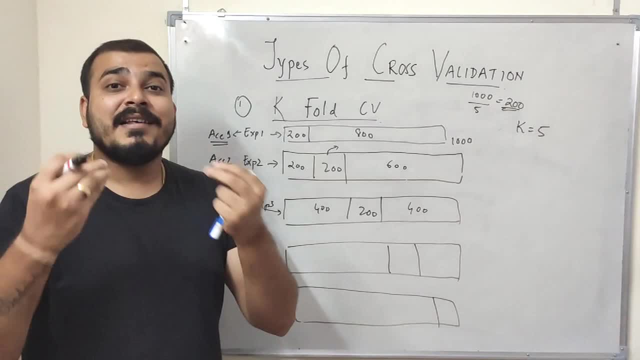 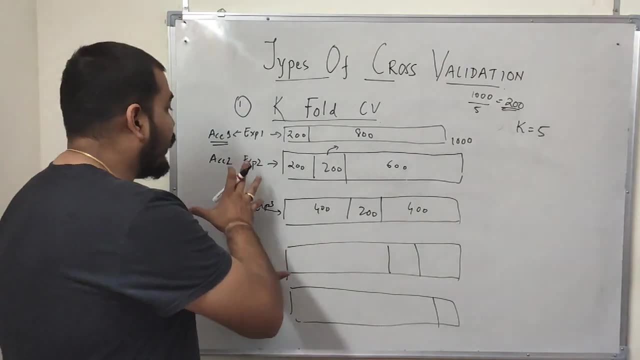 And that is how you have to talk whenever you are doing a data life projects in companies and all. I work as a data lead data scientist guys, So I am letting you know how you have to basically convey the information to the stakeholders, right? 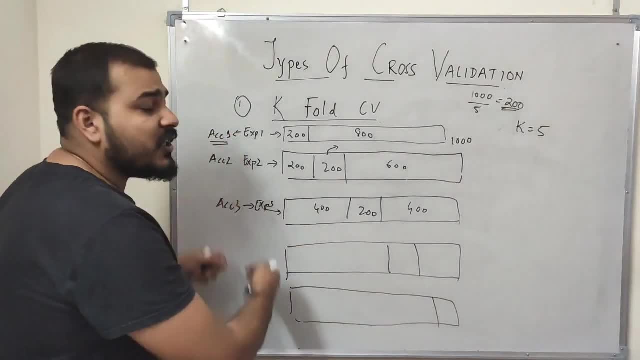 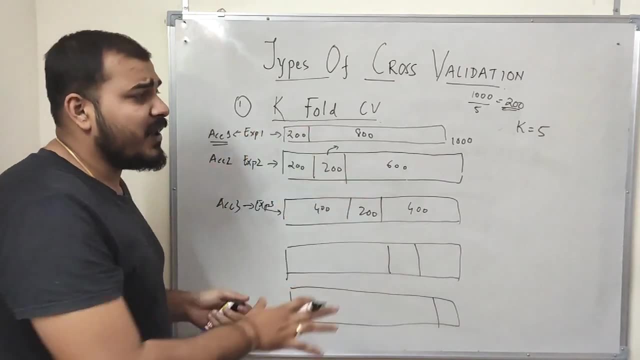 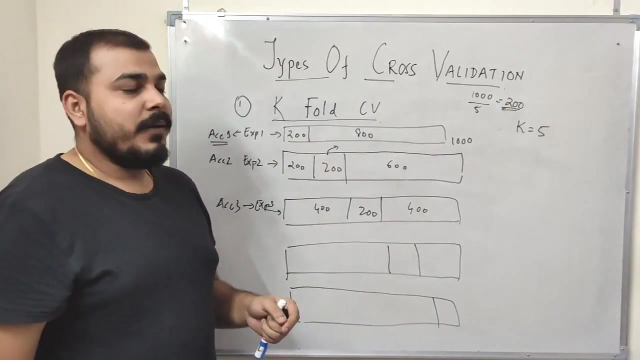 You have to basically say minimum and maximum, Or you can also say that average mean of this particular accuracy, of this particular model with respect to k-fold cross validation. Now, this is pretty much simple with respect to k-fold cross validation. There are some disadvantages in this, okay. 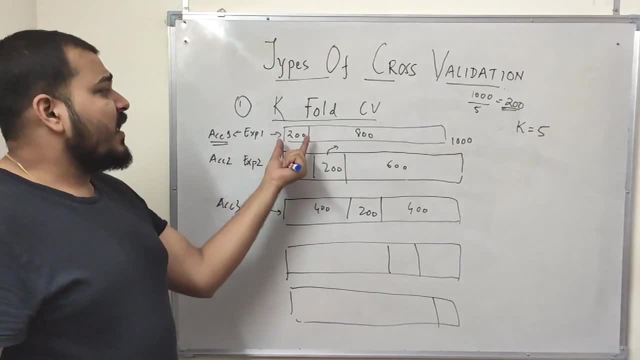 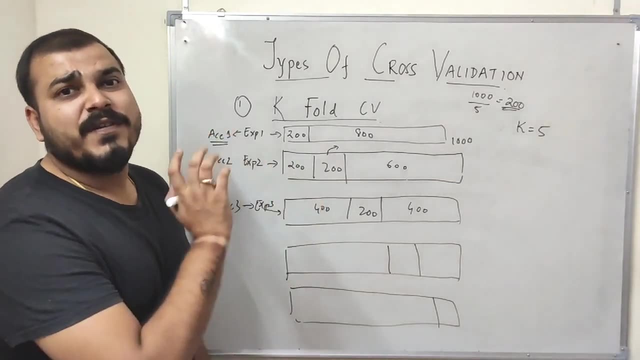 Now you can see that In experiment 1, my first 200 data set got selected as test data set. Now just imagine, in this 200 data set I have only one type of instances as my output Suppose. this is my classification problem that I am trying to solve. 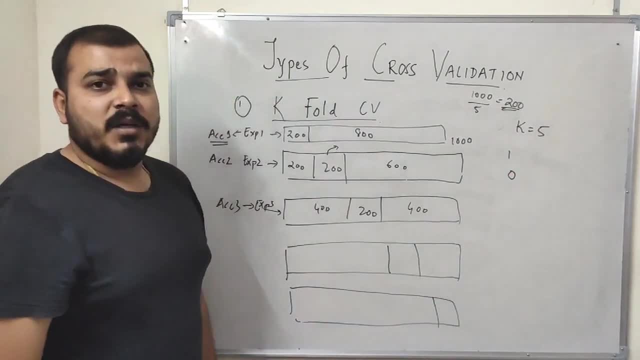 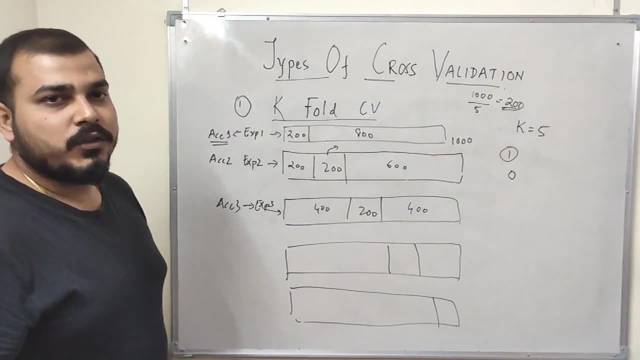 And it is a binary classification like 1s and 0s. Just imagine in the first 200 data set I had only 1s over here. okay, Only 1s over here. Or suppose in my 800 training data set, right? 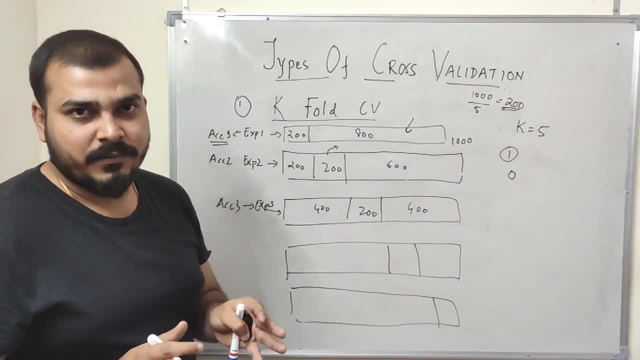 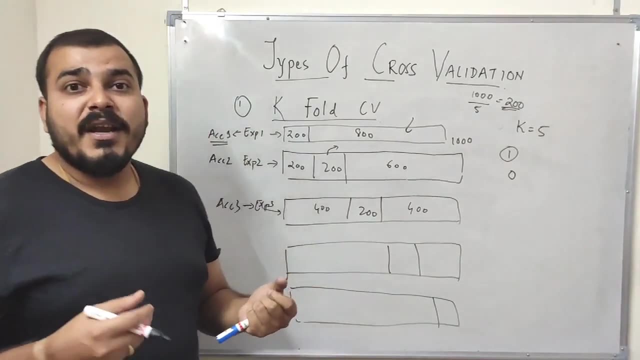 I have maximum number of 1s over here, So it becomes an imbalanced data set And that can be a problem, right? So the training that that particular model is doing, right, It may not give you the right kind of accuracy. what is actually related to this particular model? 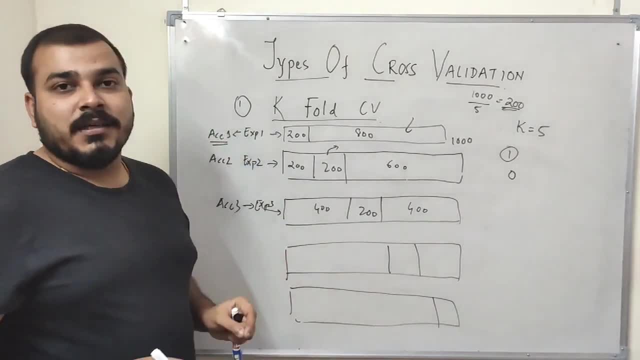 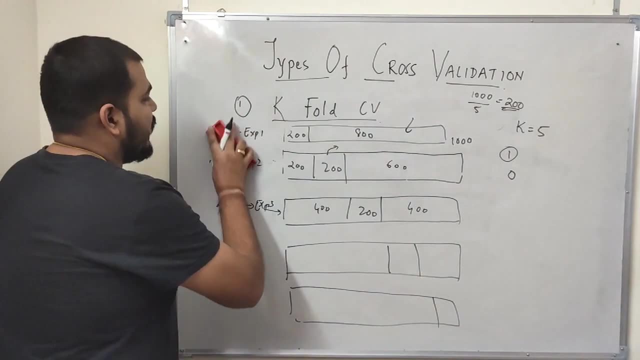 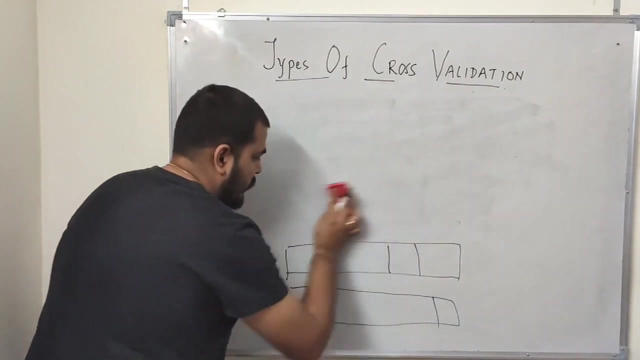 because of this particular problem. okay, So in order to solve this, we have a technique called as stratified cross validation. So the third technique, or the third type of cross validation, is basically called as stratified cross validation. I am just going to rub this. 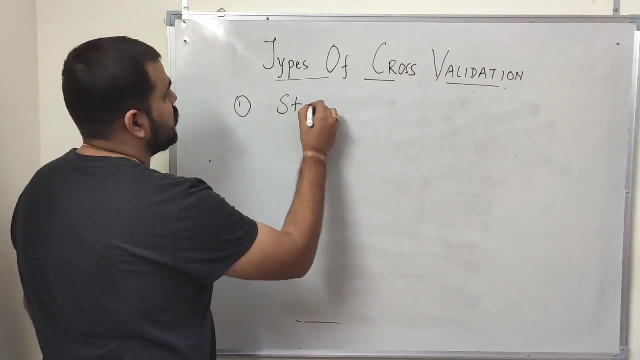 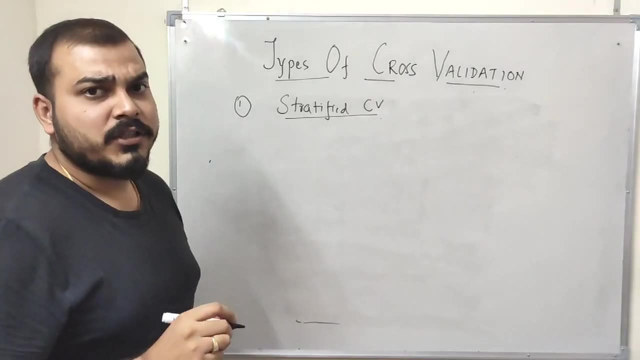 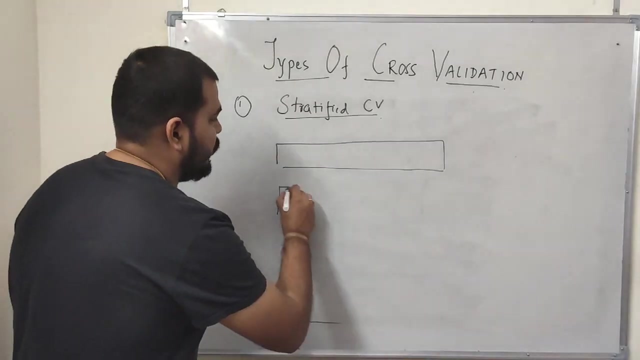 So the third technique is basically called as stratified cross validation. Now, in stratified cross validation also, everything will be same right, Everything will be same Like. suppose I have 5 experiments to perform. Suppose I am just considering 4 experiments. 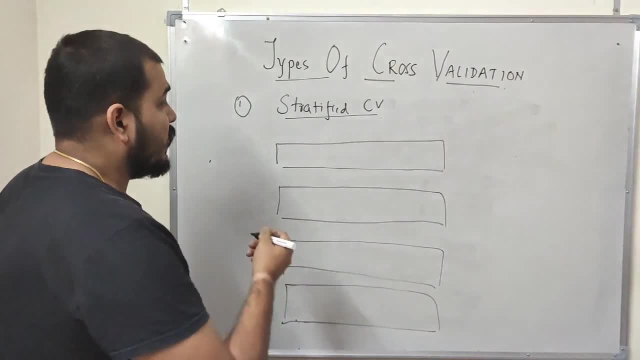 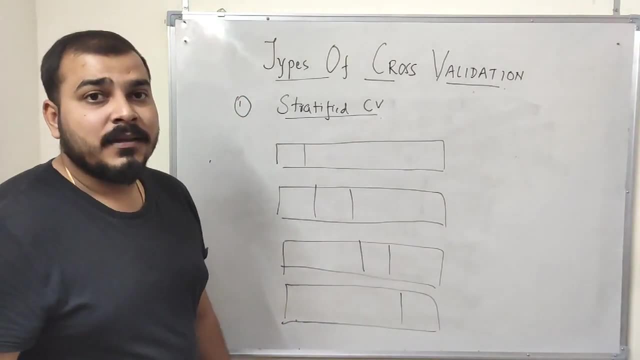 I do not have to, But I hope you are understanding what I am trying to say. So in each and every experiment, whenever the test data set is selected, it is made sure that every time the test data is selected or the training data is selected, 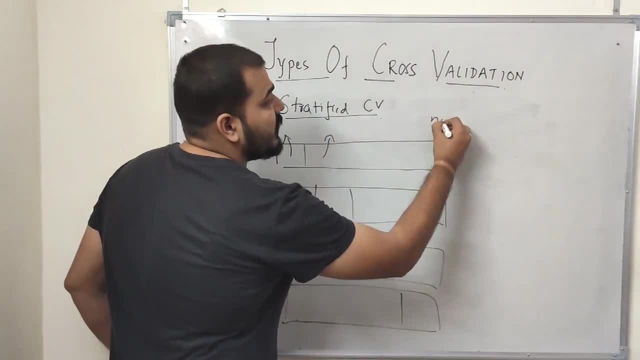 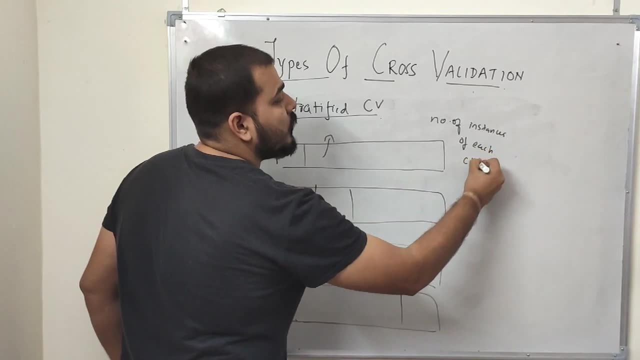 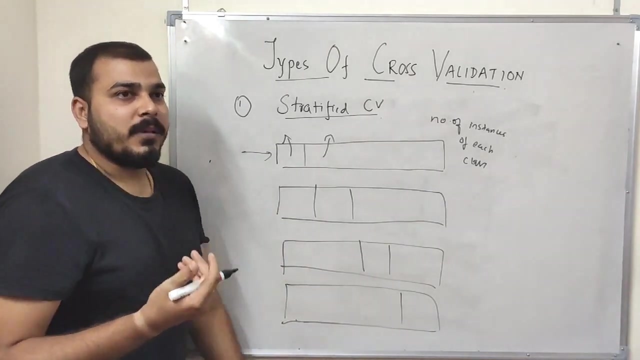 it is made sure that the number of instances of each class, number of instances of each class for each experiment in the train and test, is taken in a proper way. Now let me just give you a very good example about it. Suppose I have 1000 records. 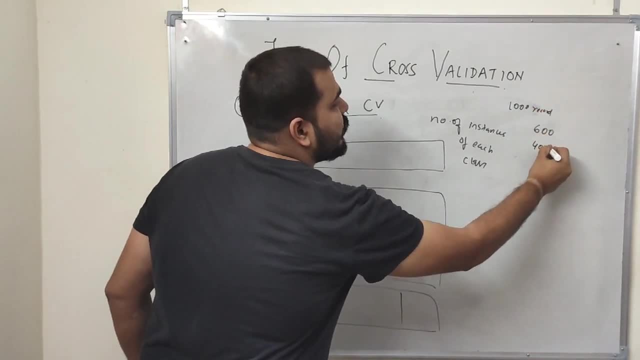 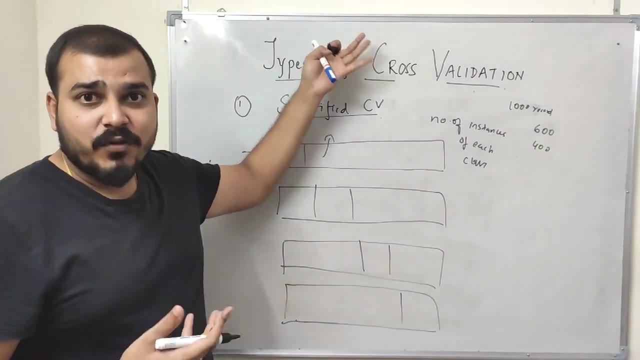 Suppose, in this 1000 records, I have 600 yes, 400 no. I am considering this as an imbalanced data set initially, guys, Okay, See, if it is an imbalanced data set, we have to fix that problem, first of all with the help of feature engineering. 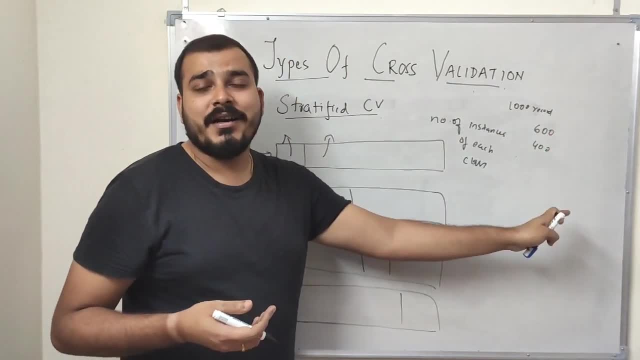 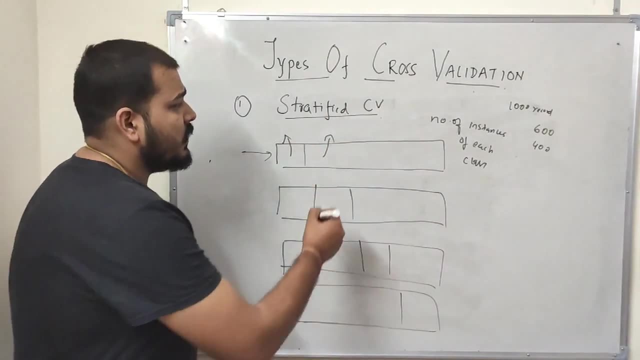 But suppose after fixing it you have got 600 records as yes and 400 records as no. Okay, Now in this case, what stratified cross validation will do in your training data set? at least it will have a good proportion of yes and no's. 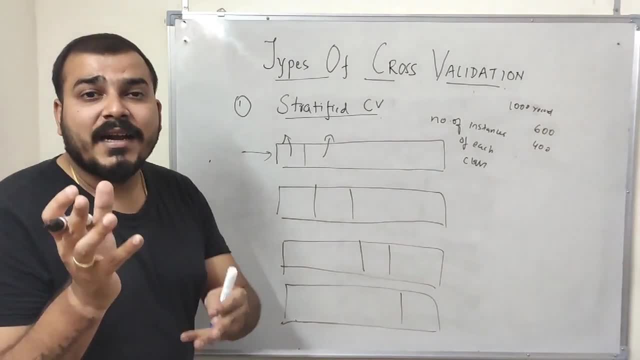 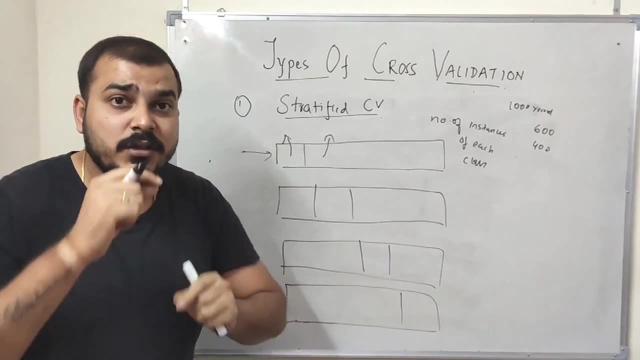 And in your test data set also, it will have a good proportion of yes and no's So that your model will be able to give a good accuracy for that. Okay, And understand why stratified cross validation is basically used To prevent the disadvantage that was present in cross validation. 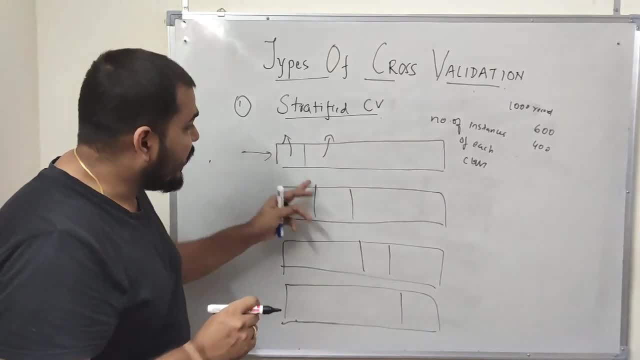 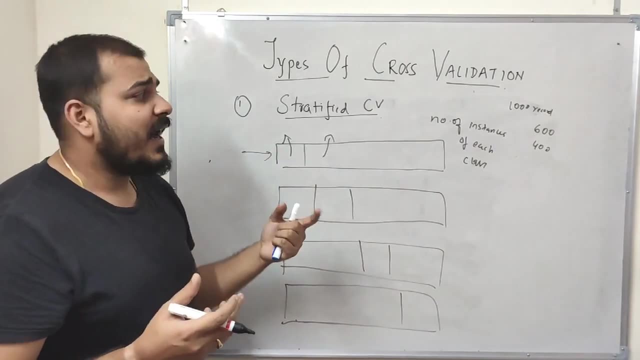 That is basically k-fold cross validation. So in each and every experiment it will make sure that the random sample that is basically populated in train and test will be in such a way that at least some number of instances of each class will be present in through that. 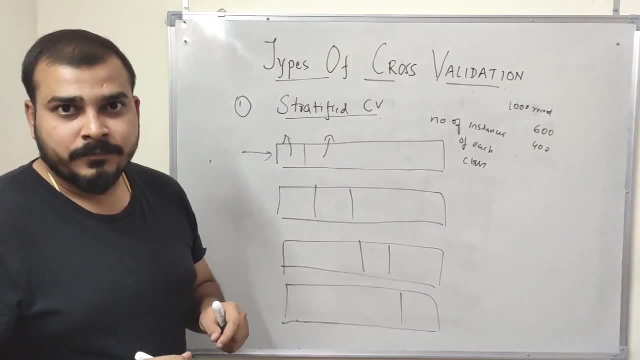 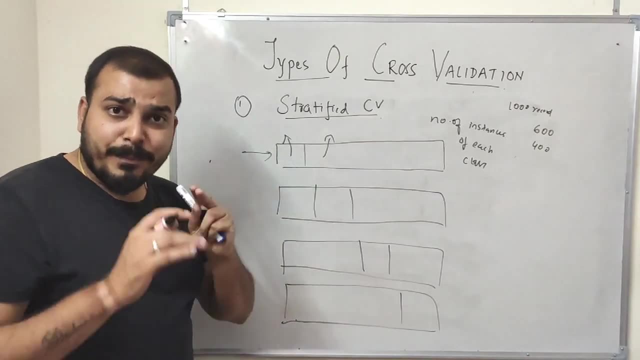 And that is how that problem of k-fold is basically fixed. Very simple, See, guys. in my next video I will be showing you how to perform k-fold stratified cross validation practically with the help of a very good use case from Karel. 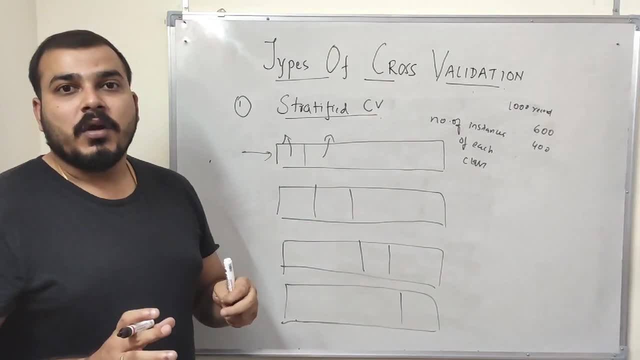 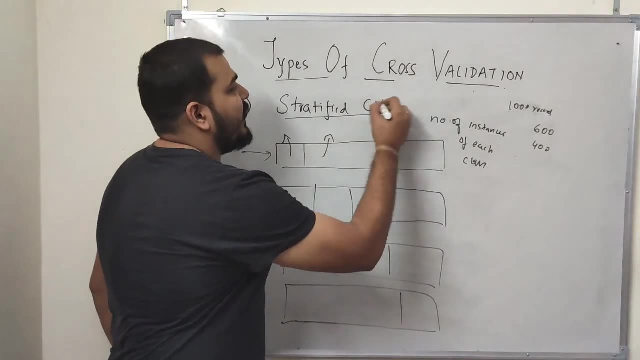 Okay, Just try to understand how this is basically done. Okay, So this is pretty much clear. So remember, in every experiment that you do- suppose you are doing- that my stratified k-fold value, k-value, should be 5.. 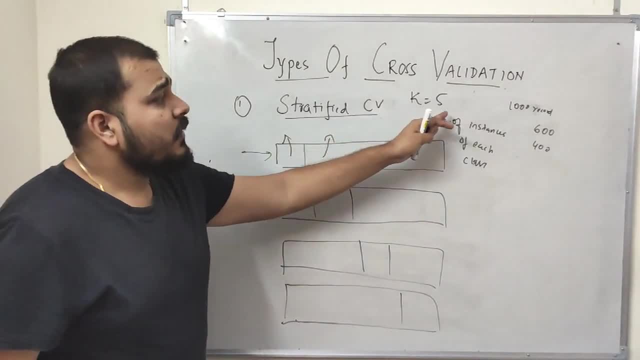 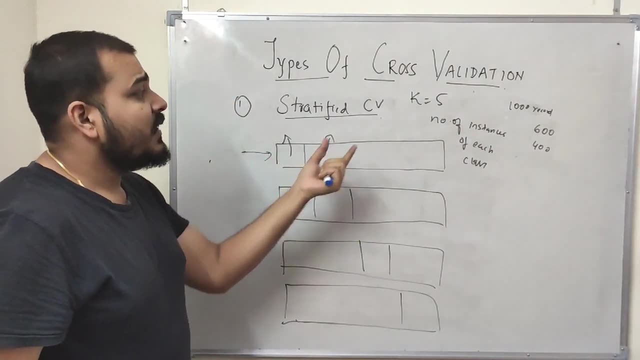 That basically means 5 experiments. So 5 divided by 1000 will be 200.. So this 200 data set for test will be selected in such a way that proper number of instances of both class. What will be the percentage? It depends on this particular data set, guys. 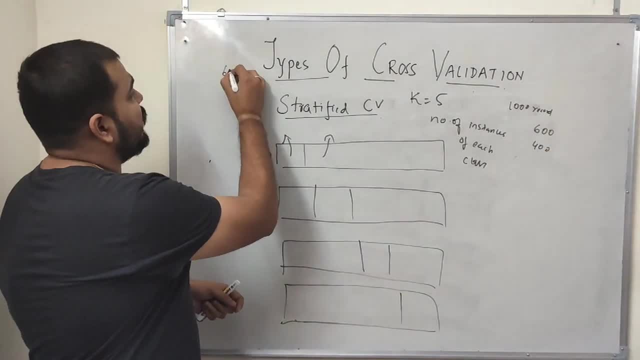 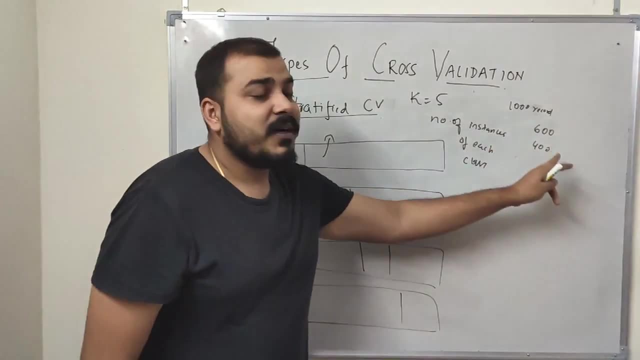 But it will make sure that at least 60-40,, 60%-40% is there, Or at least 70-30 is there. Okay, But it completely depends on this particular data set. also Okay, But again, if the data set is completely imbalanced, 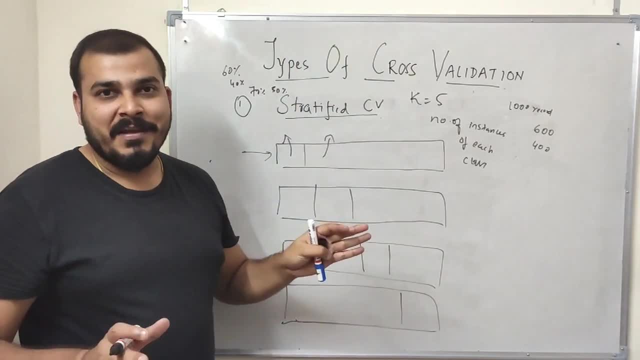 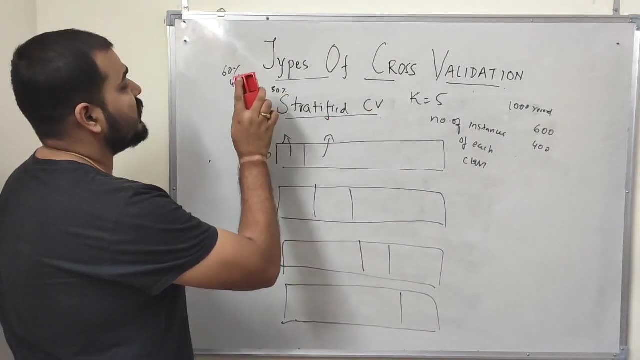 you have to fix that from starting, That nobody can help. Okay, And that is why we do feature engineering. Yes, So this was the second technique. Now the third. sorry, this was the third technique. I am going to discuss about the fourth technique. 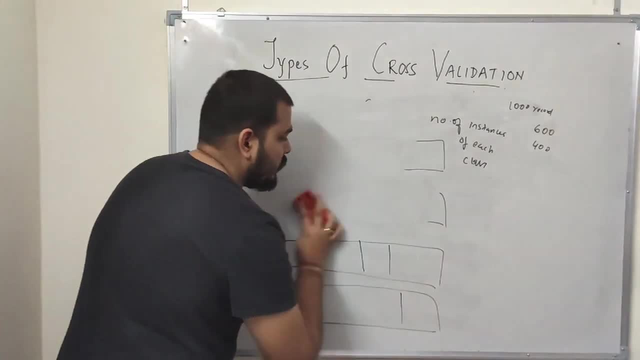 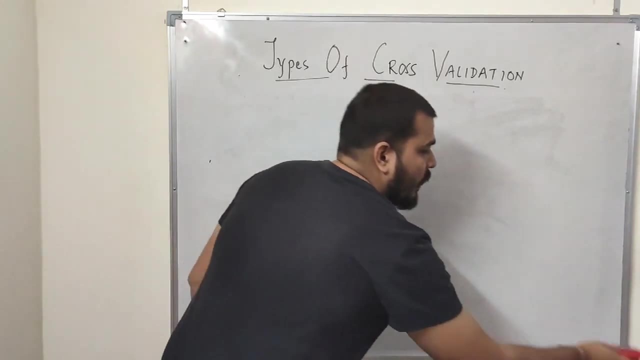 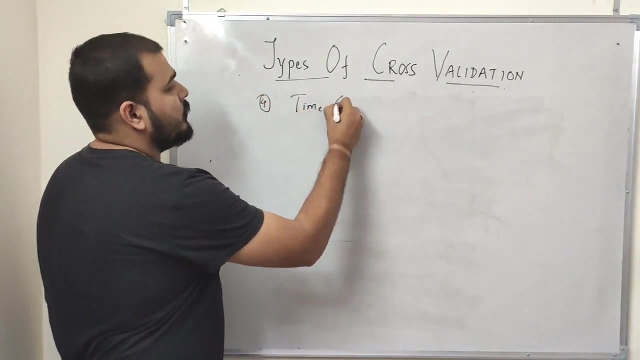 which is called as time series cross validation. And this is the last technique, And time series cross validation works for a completely different problem, guys, Suppose, if I take an example of. so the fourth technique is basically time series cross validation. Time series cross validation. 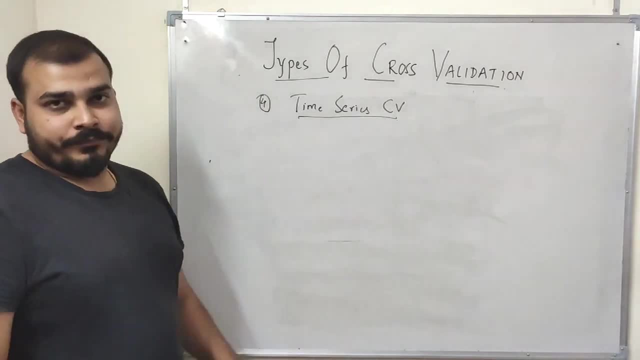 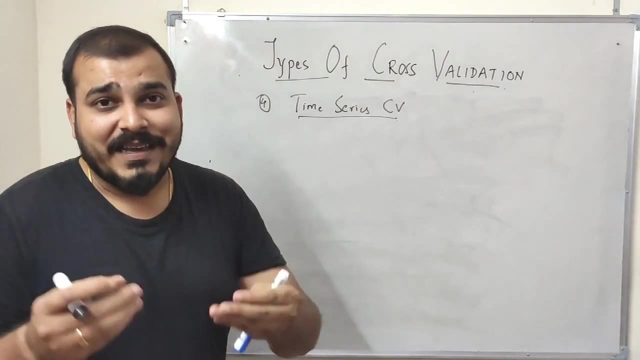 Now where it will work. Whenever you have a data set of time series kind of type it is, just think over it- Can you split that based on your date? See if you have a training data set and some test data set. 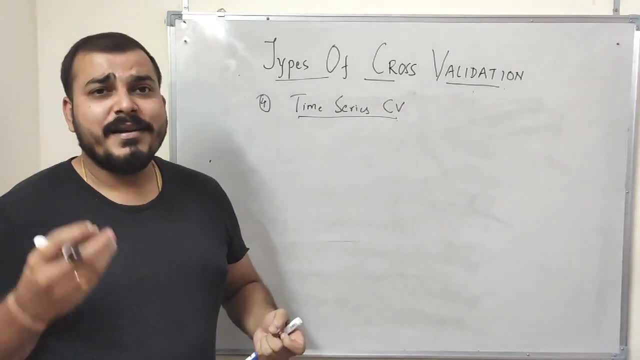 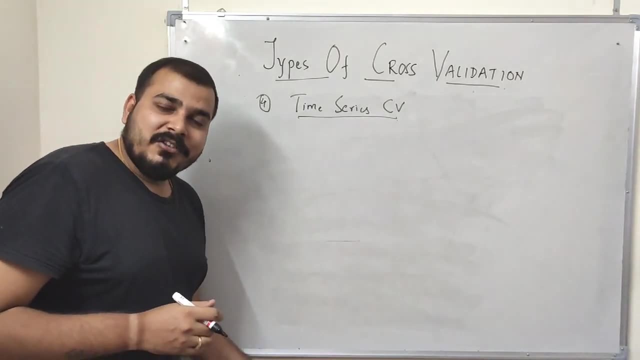 or if you have a data set that is related to time series problem. Let me just give an example. like stock price detection Now in stock price you have to predict the future data Right. So to predict the future data, you cannot do a train test, split and try to find out the accuracy. 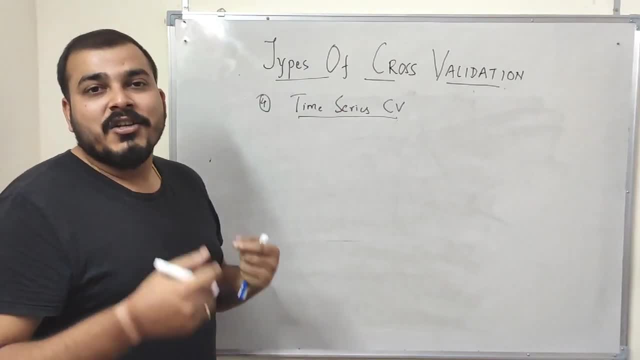 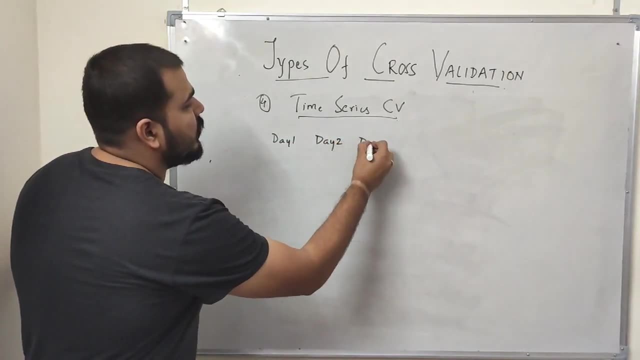 Because that data is based on time series, Right? So in that case, what we do is that suppose this is my day one data, day two data day three data. Okay, What suppose? first of all, I am doing this? 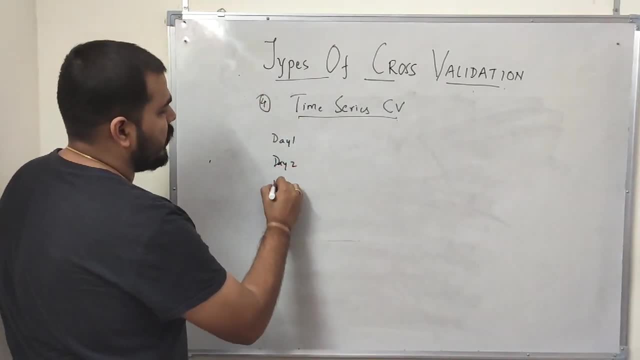 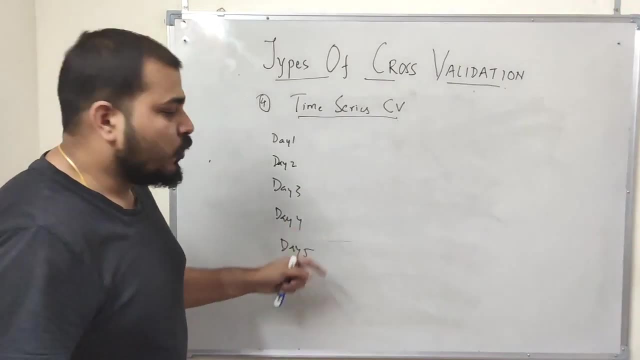 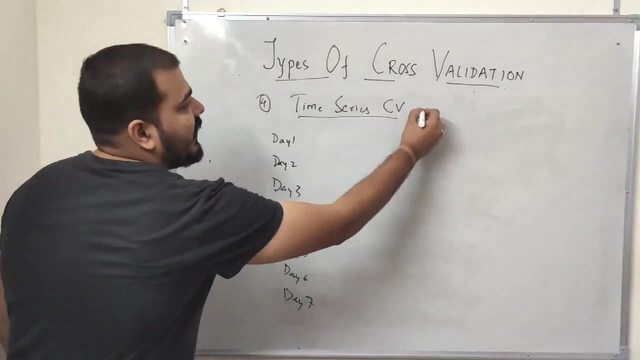 Suppose I have day one data, day two data, day three data, day four data and day five data. Okay, Now we need to do the prediction for day six, day seven and future of like this: Okay, And these are some values. 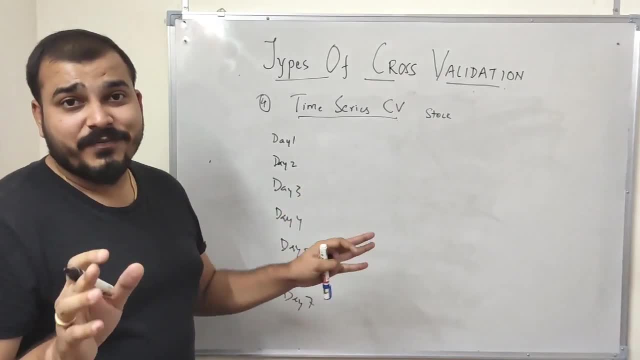 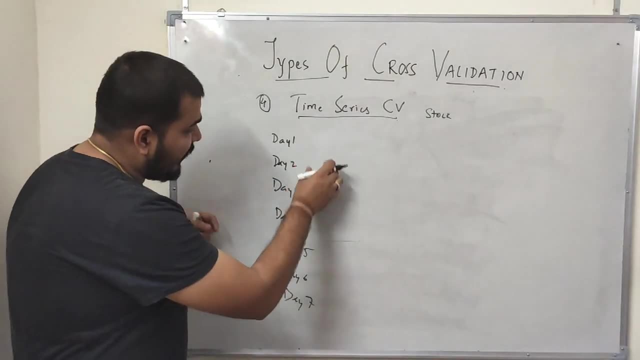 I am taking example of stock And, guys, if you are not seeing my stock prediction video, I have already made on that And there we have actually performed time series cross validation. Okay, Now this is day one, day two, day three: 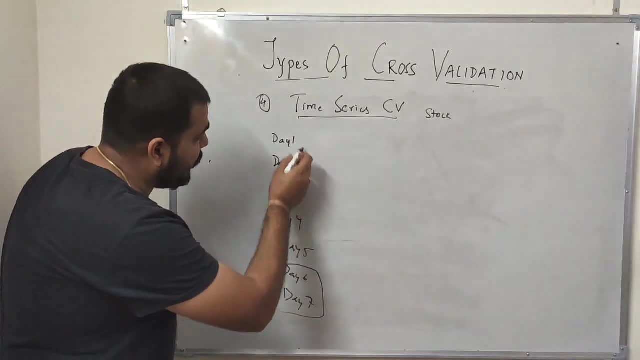 day four, day five, day six, day seven. I want to find out day six and day seven output. Okay, So I have to be dependent on this particular data itself. So what we do is that, by using time series, cross validation. 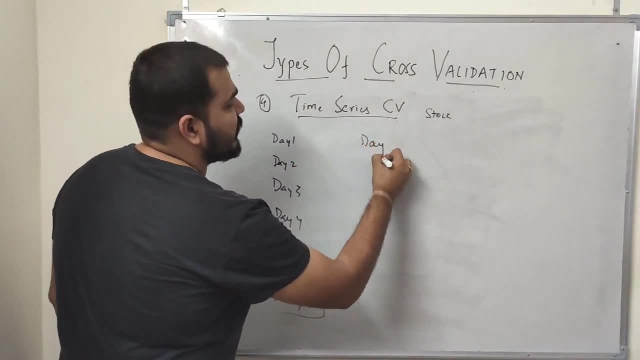 first of all, I will change the data structure like this. It will be day one, day two, day three, day four, day five. So the first, first row of my data will be like this, And when I say day one, 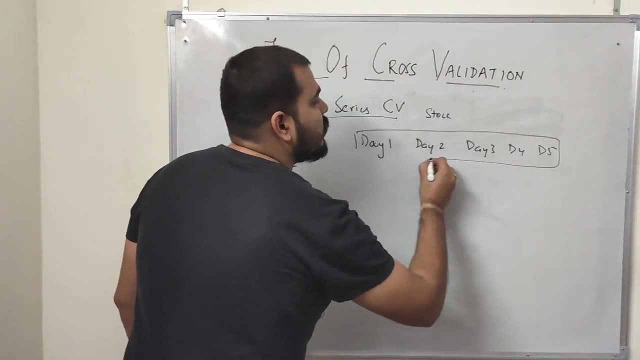 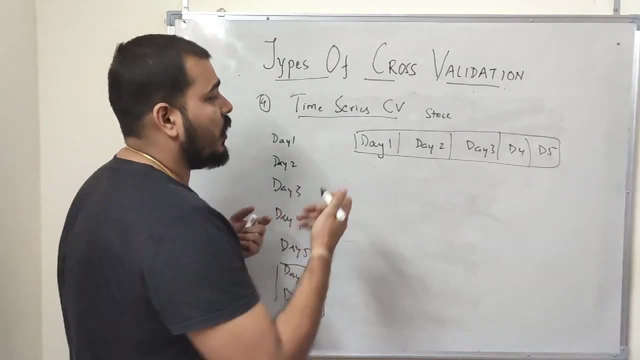 day two, day three, day four, day five. it will be day one, day two, day five. These are the basic information about the stock price. Okay, Now I want to predict the price of day six, So day six will be my output. 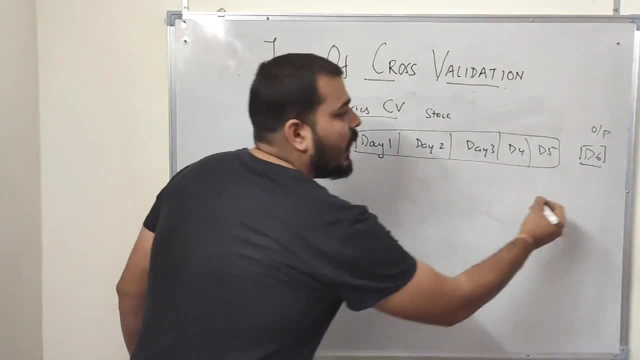 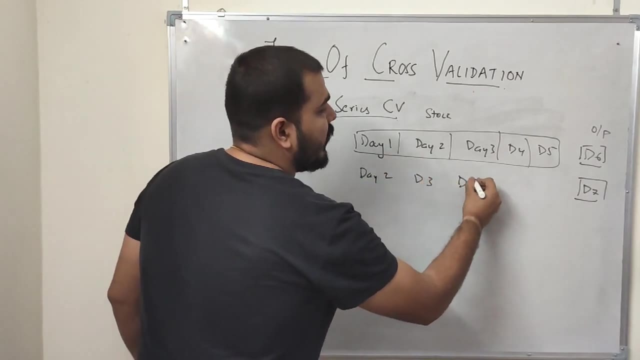 Okay, And now. similarly, I want to calculate the output of day seven. So what will be my input data? It will be basically day two, day three, day four, day five and day six. So this is how I will create my records. 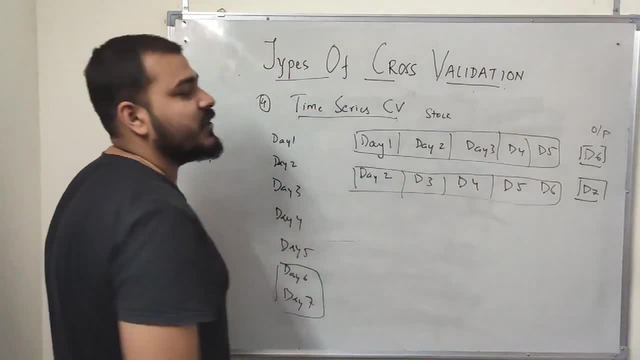 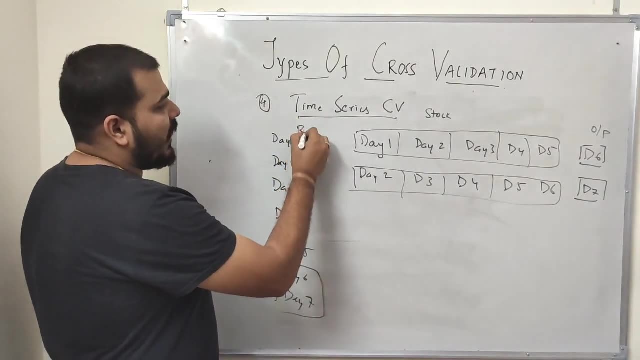 This is how. this is how my time series cross validation will be- series cross validation work, and this you have to do for time series data. you can't help it out, you know, because this is the structure. suppose you are using an RNN LSTM model, so at that time you will be performing this kind of data. 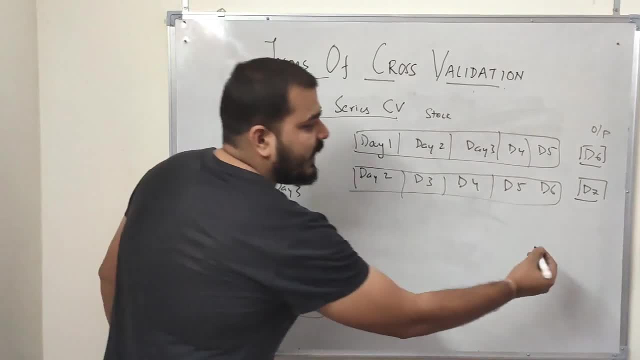 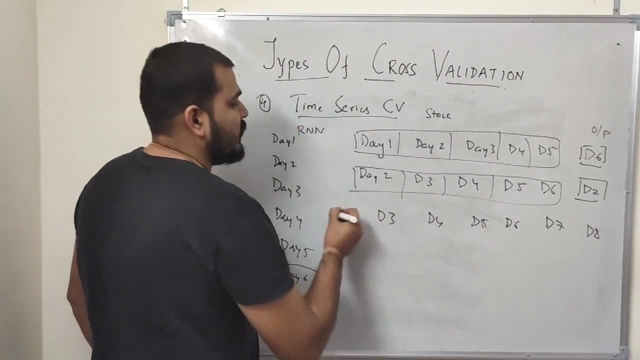 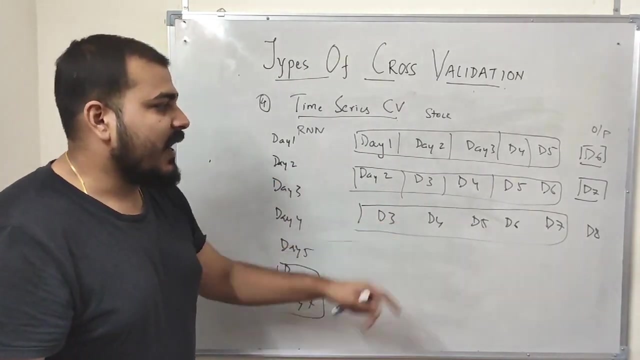 preprocessing and you'll be creating this kind of records now. similarly, if you want d8 output, that time you will be creating d7, d6, d5, d4, d3. this will be a third record and that is how it will continue on going on now. after that, what? 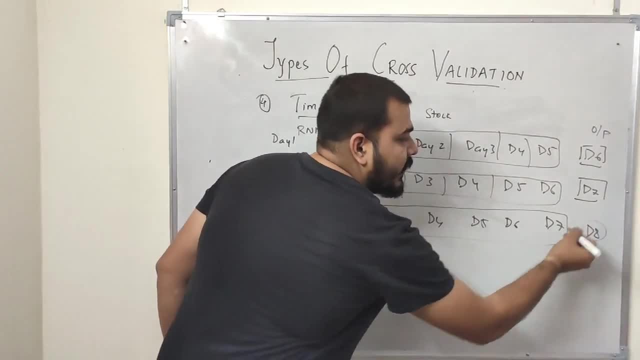 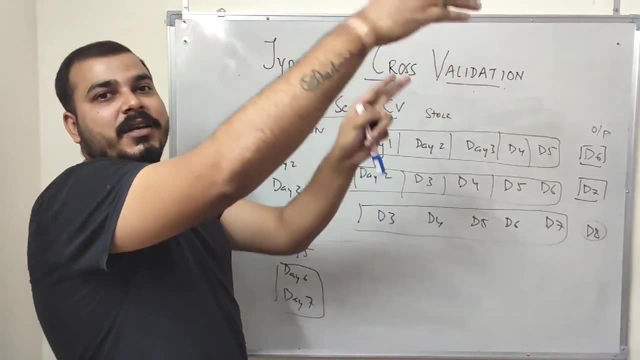 will happen for day 9, day 10. so at that time, suppose you have calculated d8. right now all you have to do is that shift this one step up, take d8 and calculate for d9, and that is how the stock prediction will be calculated. 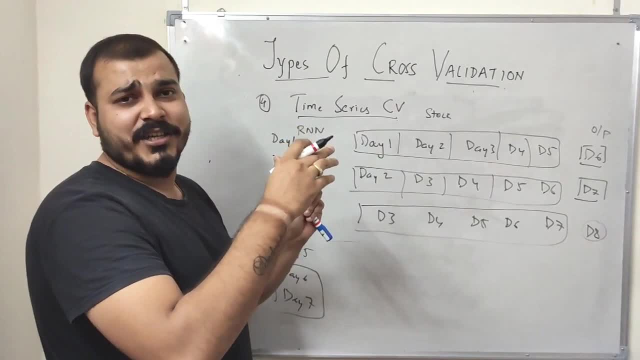 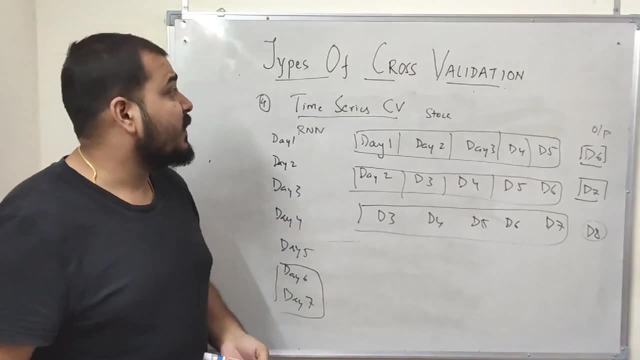 time series calculation- let it be sales prediction, let it be stock price prediction, and it can be implemented for various things, and that is how time series cross validation works, guys. so I hope you liked this video. please subscribe to my channel and hit the bell icon so that you don't miss my next video. 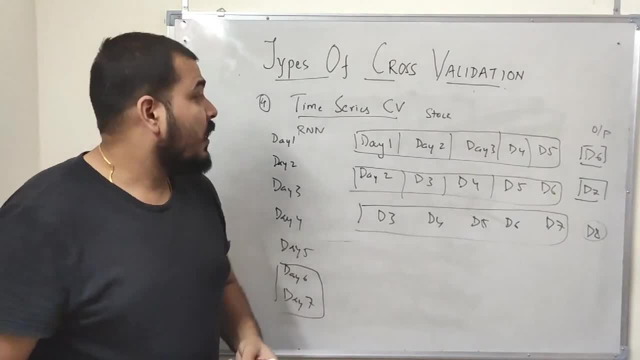 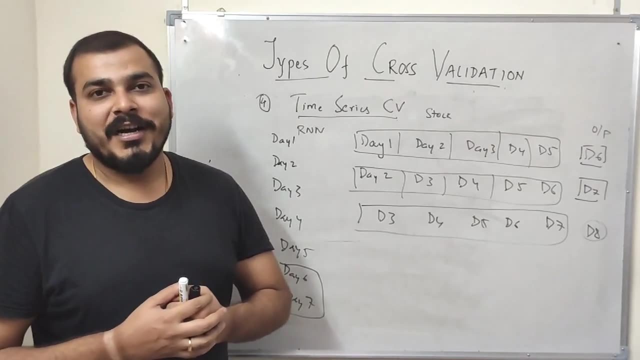 this particular video, you understood what are the different types of cross validation. please do subscribe the channel if you have not already done. please share with all your friends. I'll see you all in the next video. have a great day. thank you one and all. god bless you.